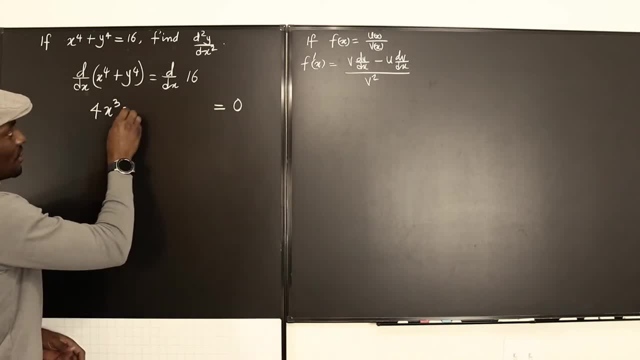 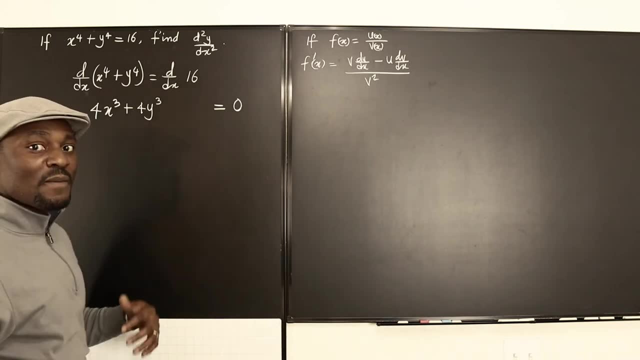 the fourth is x to the fourth. Okay, How would you differentiate? Okay, you're just going to say plus 4y to the third, But this is y and this is not x. So you have to do the chain rule. You know, you have to differentiate y itself. And when you differentiate y itself, 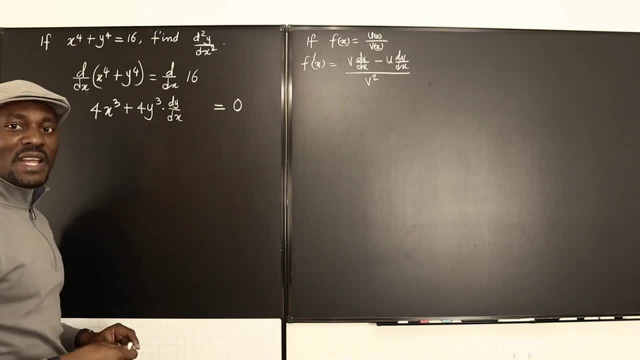 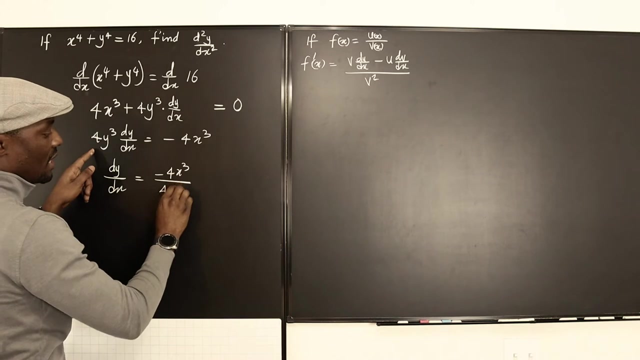 it's going to be dy dx And that's where dy dx comes from. So now let's isolate dy dx. We're going to have 4y cubed. dy dx equals negative 4x cubed. And then we have dy dx is equal to negative 4x cubed over 4y cubed. It gives. 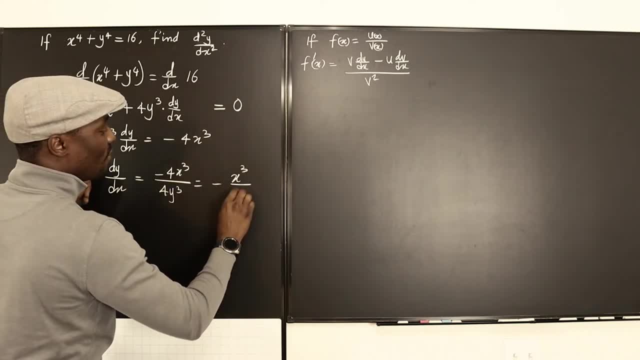 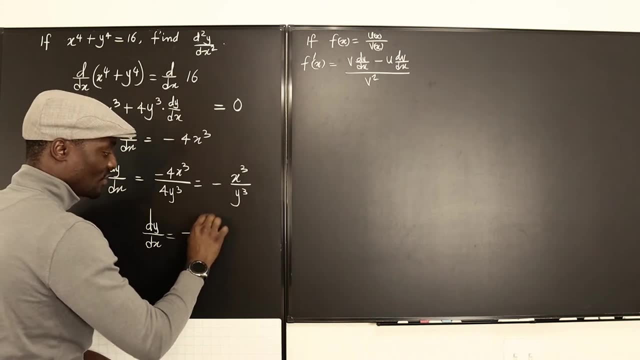 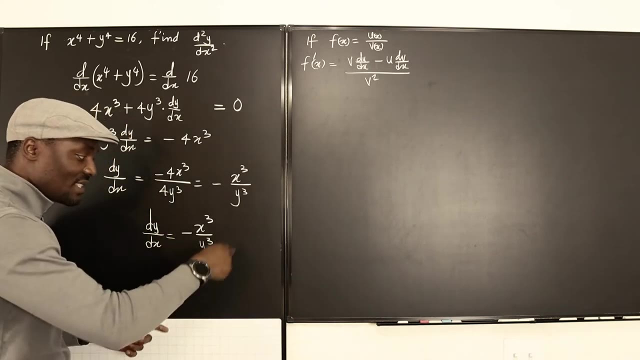 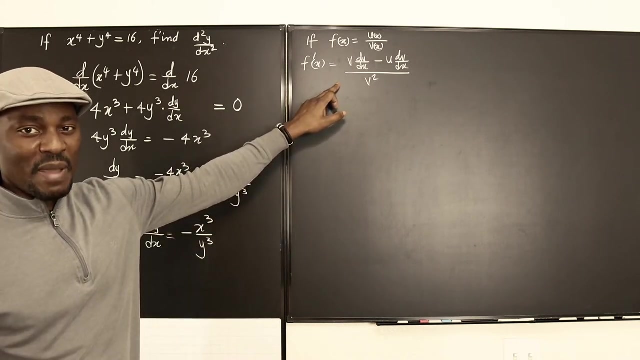 us negative x cubed over y cubed, And that's it. dy dx equals negative x cubed over y cubed. We just need to differentiate this one more time Now, because this is a quotient. we're going to supply the quotient rule. The quotient rule is what you have, right there, Remember. 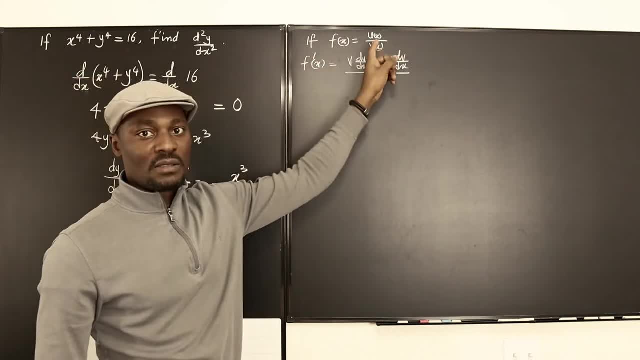 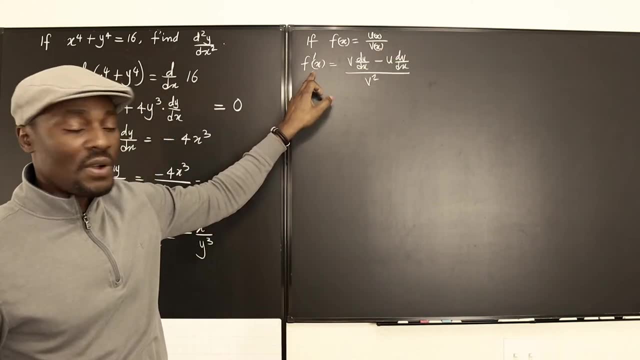 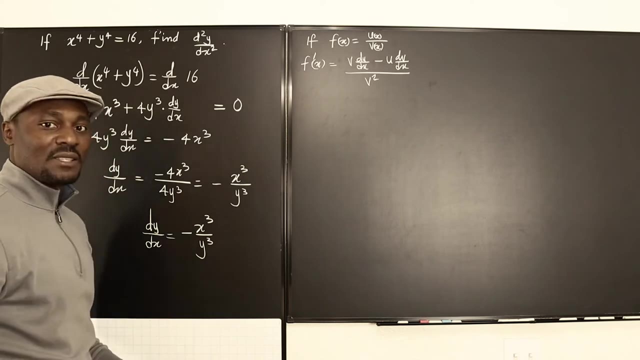 that if a function is a quotient, that is, the numerator is a function of x, the denominator is a function of x, then the derivative of that function, like we have here, is going to be v, du, dx minus u, dv, dx over v squared. Apply it to this, Doing implicit differentiation. 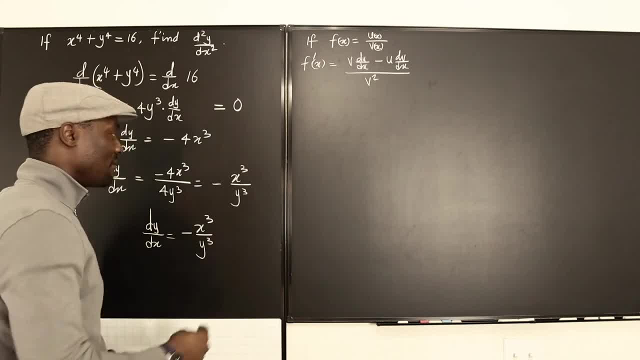 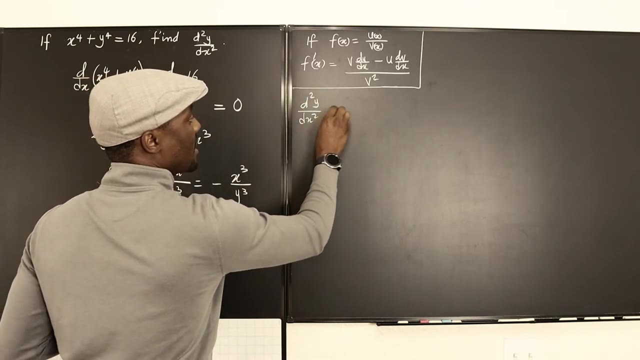 also it needs to be much cleaner. So let's do that. So, applying this we're going to have, the second derivative will be d2y dx squared, So d2y dx squared will be equal. to remember, this will be our v, so that will be y cubed. 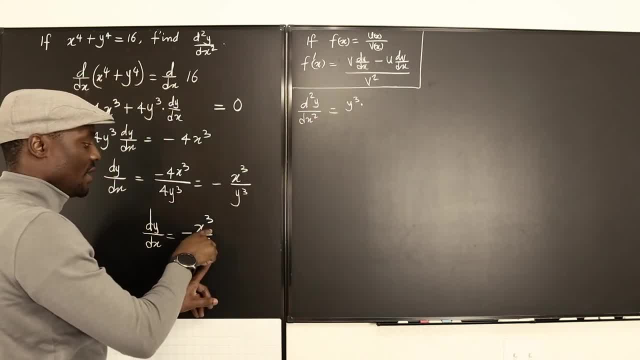 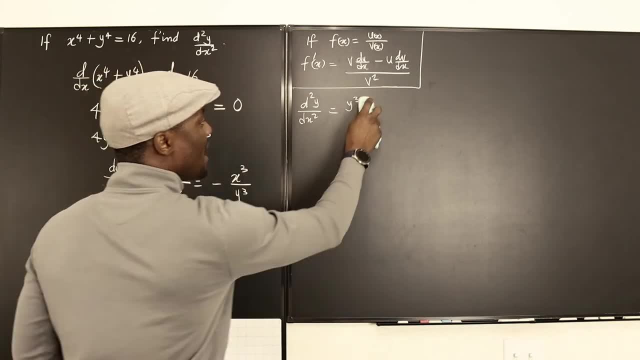 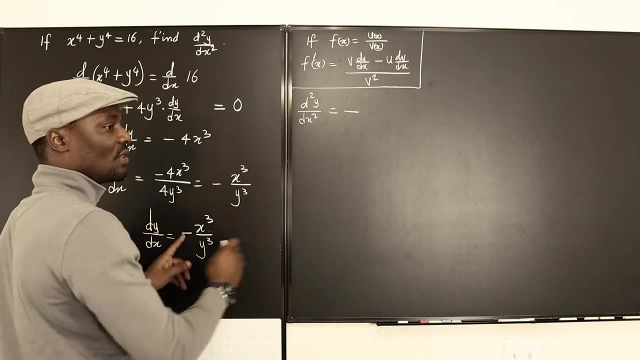 multiplied by the derivative of the top, which will be 3x. What do we do to the negative sign? OK, Let's not throw the negative sign away, So I'm just going to leave it on the side here along this line, and then we do our calculation. 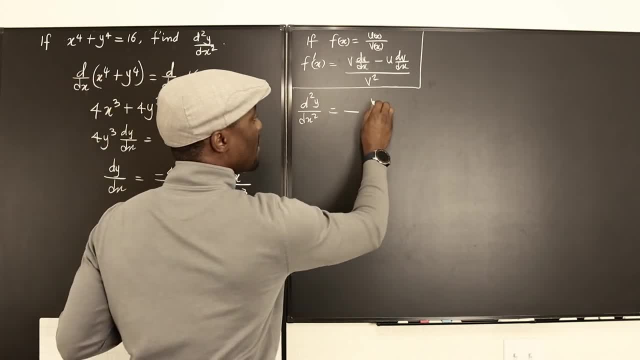 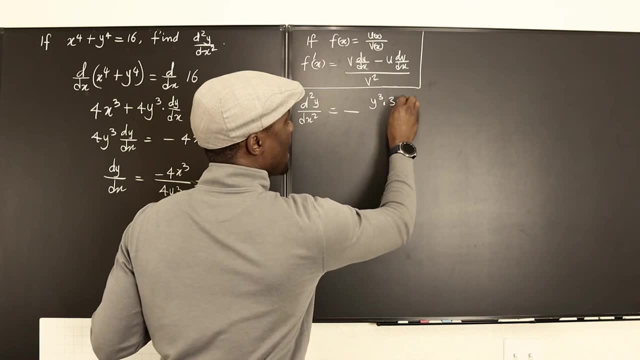 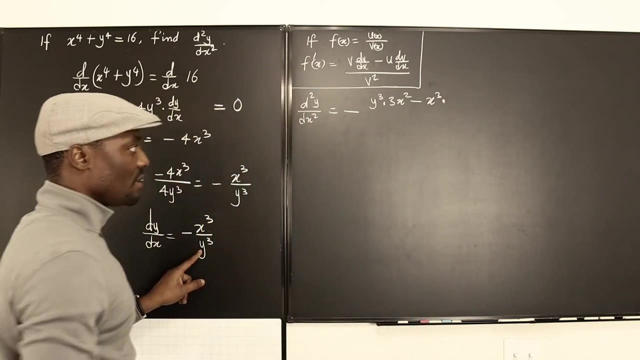 without using it. Let's just leave it the way. it is OK. So we're going to have y cubed multiplied by the derivative of this, That's going to be 3x squared times 3x squared, minus x cubed. multiplied by the derivative of the bottom, That's going to be 3y squared dy dx. 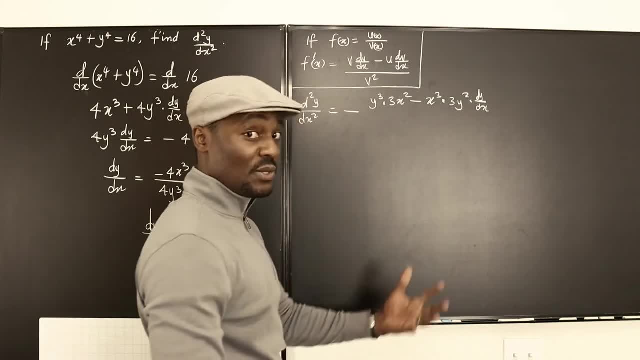 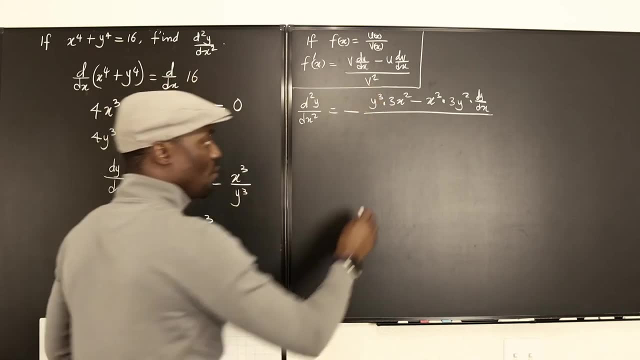 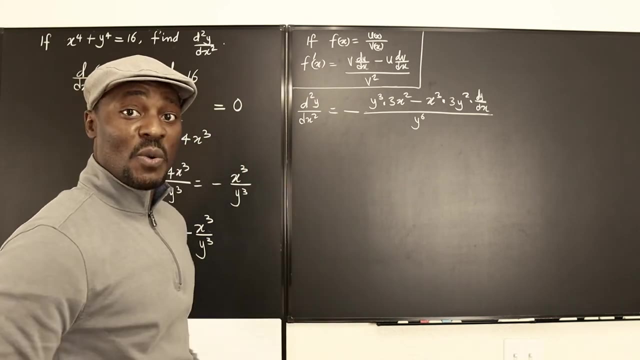 And don't forget, every time you differentiate the y, you have to multiply it by dy, dx, OK, And all of that divided by this square, The square of y cubed, will be y to the sixth. OK, Now, this is it. We just need to collect like terms and do what we need to do. However, 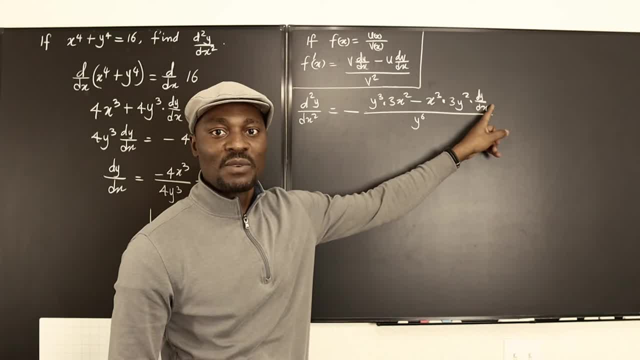 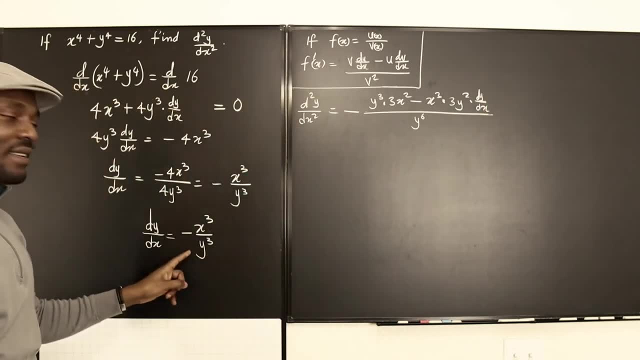 there's something here: dy dx. We're not looking for dy dx, we're looking for d2y dx squared. So what is dy dx? dy dx right there. So let's just take this entire term and put it here and see what. 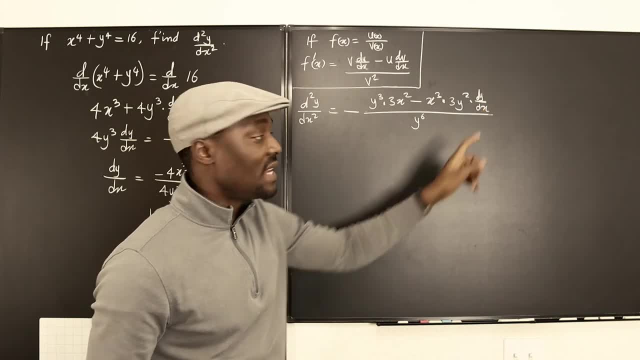 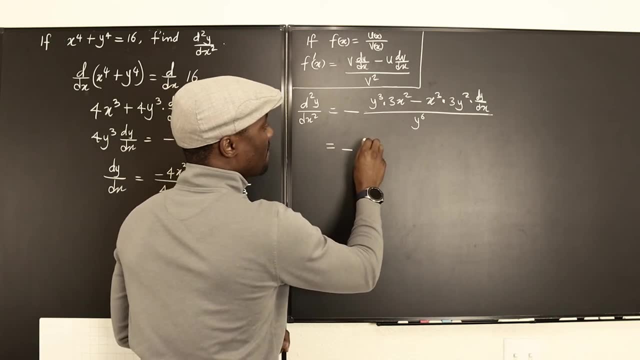 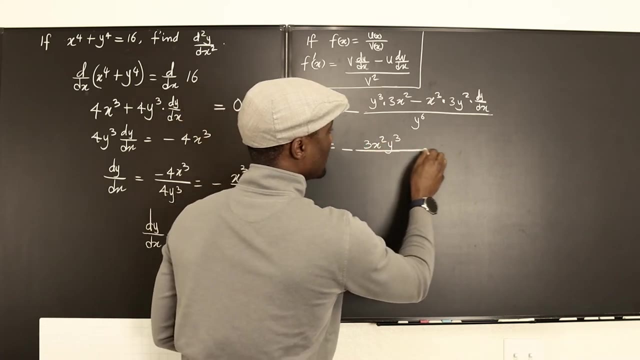 it's going to do to this term, because you're multiplying this term by dy dx. So this is going to be. we'll still leave the negative sign. All of this will become 3x squared, y cubed. OK, Show the line Minus. see, I'm still ignoring the negative sign. we're going. 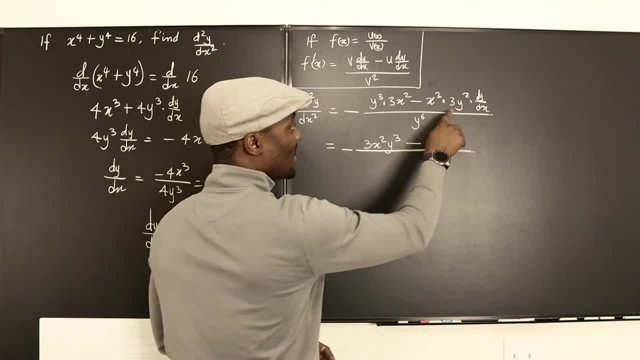 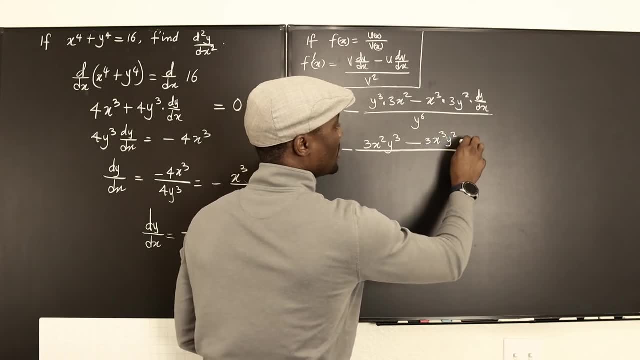 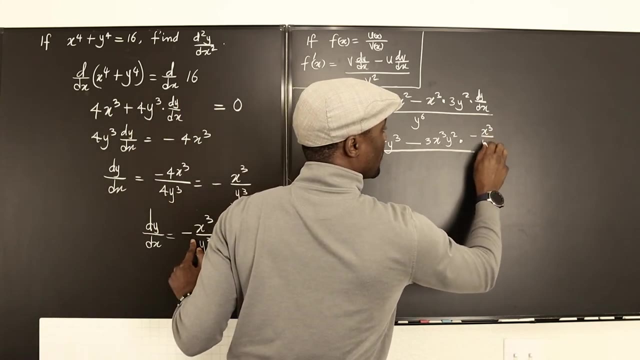 to use it later or we'll never use it. Let's see, Let's see. So this is going to be 3x cubed y squared, 3x cubed y squared, multiplied by negative x cubed over y cubed. Negative x cubed over y. 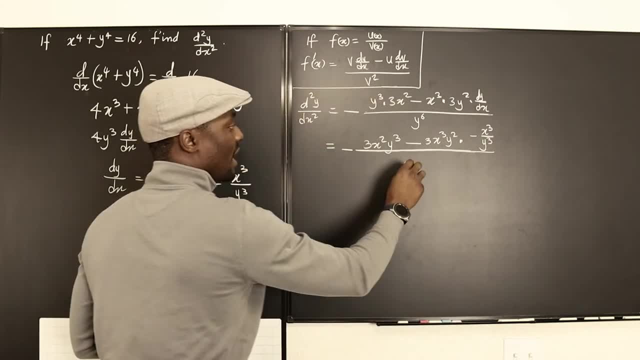 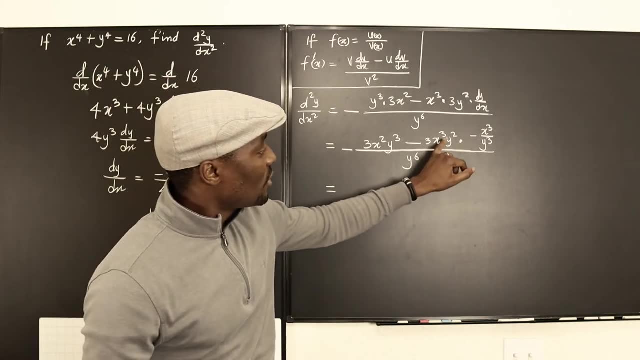 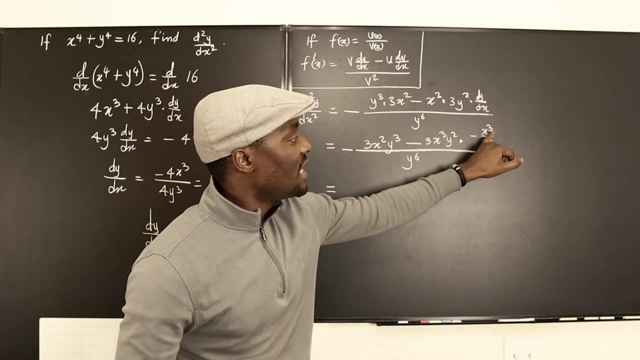 cubed, Okay. Now divided by y, to the 6th: Okay. This is where your algebra skills will show up. Now, remember, when you multiply this by this, this y squared will cancel two of these and you have one left. Okay. And then this negative is going to change this to a positive. So the next line: 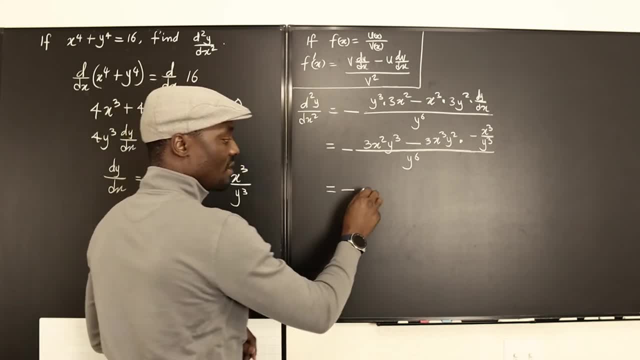 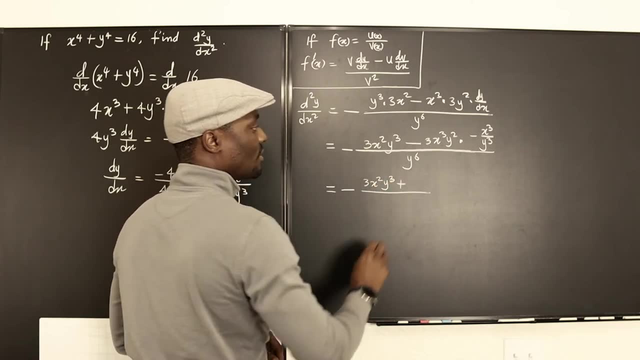 you have is going to look like this. You'll still have your negative here, Okay. And then this is going to be 3x squared y cubed. This becomes plus. Okay, This x cubed multiplies this. It becomes 3x squared y cubed. 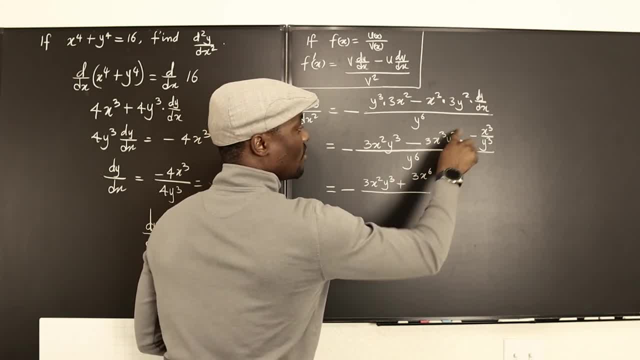 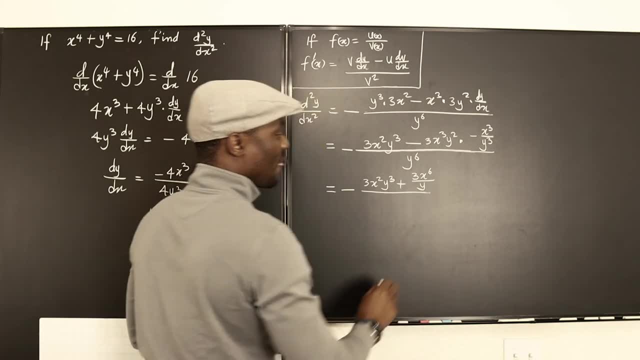 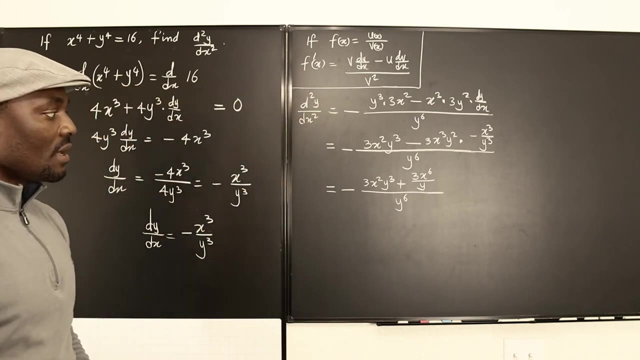 x to the 6th, This y squared is canceled. two of this: Oh, that's all you have. 3x to the 6th over y. Ah, Divided by y to the 6th. Okay, So what can we do? We can actually get rid of this y by multiplying. 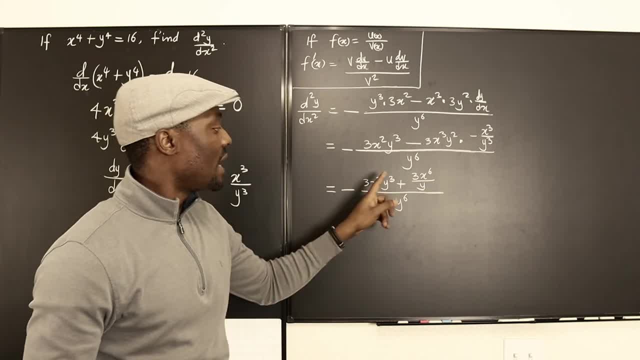 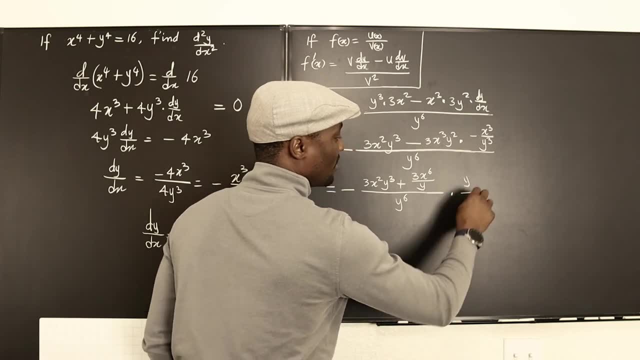 each of these terms by y. Okay, If we multiply this by y, this by y, this by y, we do that. by doing this, We can say y over y. Okay, We just multiply. That way, this y will take out this y, but it will multiply. 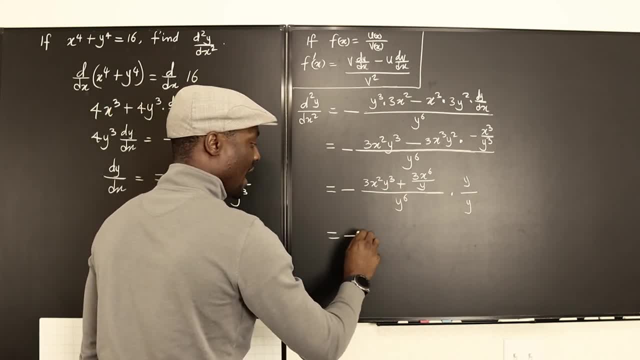 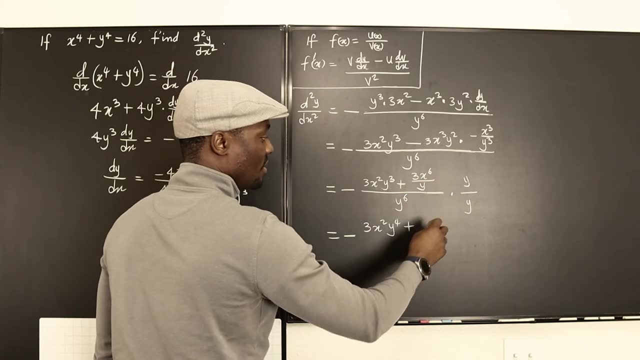 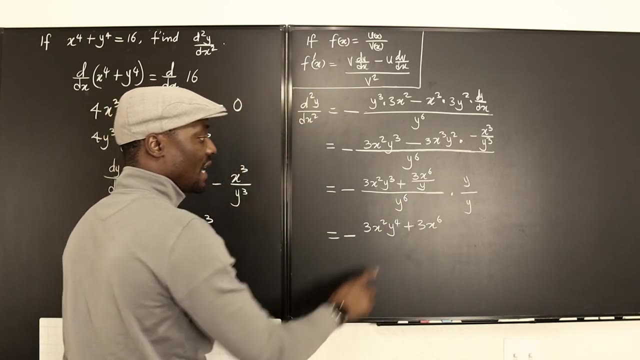 this y, It becomes y to the 4th. So your answer is now negative. You have 3x squared y to the 4th, plus what's left here is just going to be 3x to the 6th, because this y will be gone, multiplied by that. 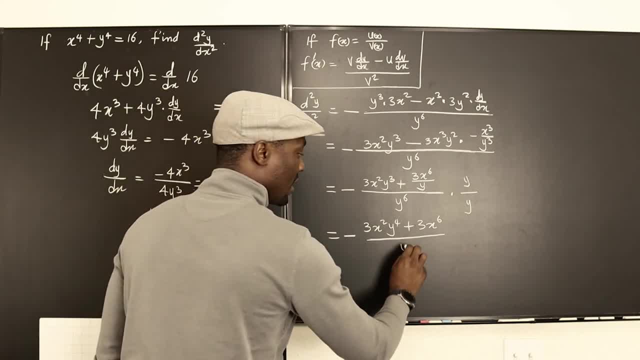 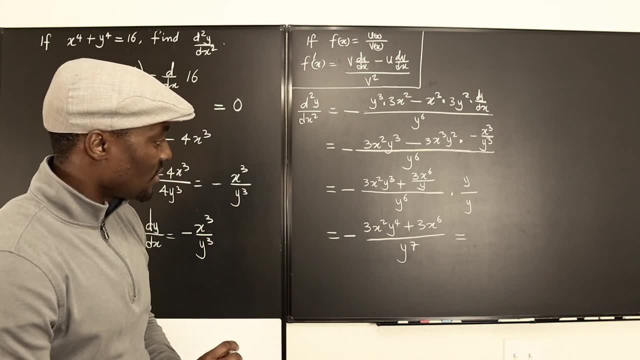 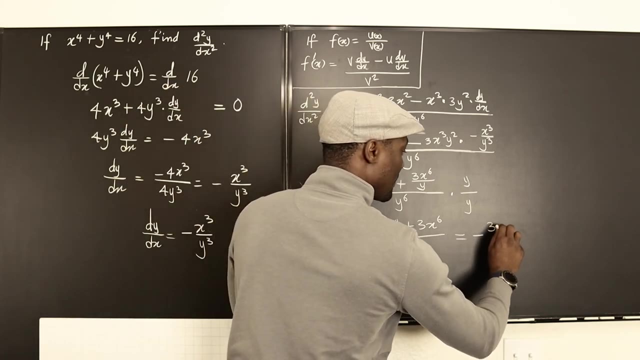 And this becomes y to the 7th, y to the 7th, Which will be equal to. let's just collect the factors that we can take out. We can take out 3x squared Okay, So that's going to be negative. 3x squared into what is left will be y to the 4th plus. 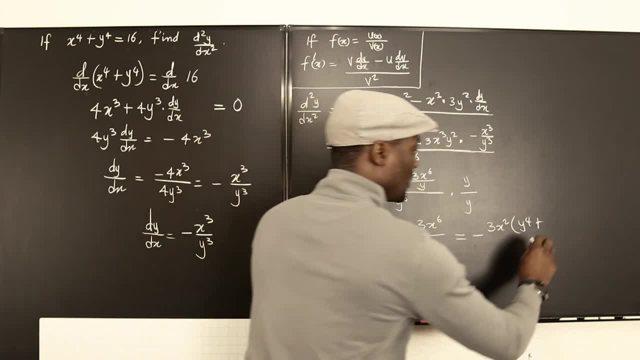 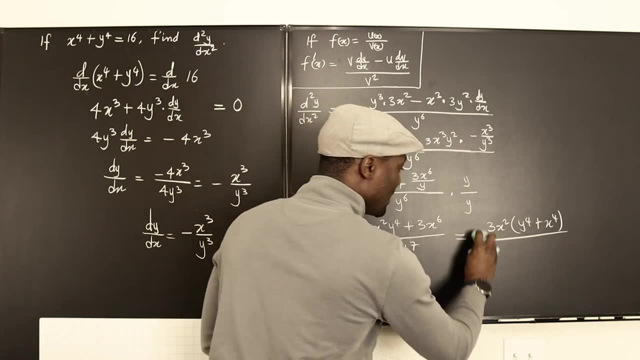 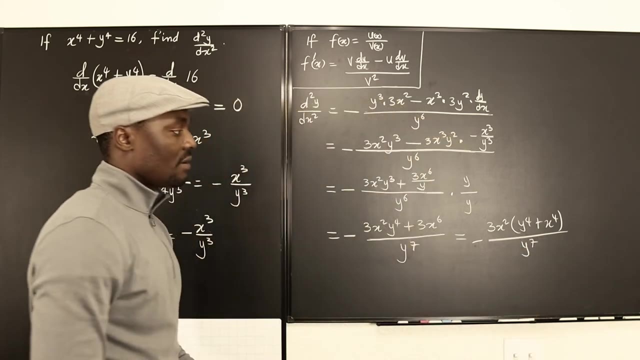 to take out 3x squared, we have x to the 4th. Ah, interesting Over. oh no, that negative belongs to the middle line. Okay, Don't lose it Over. y to the 7th. Okay, We're done with our calculation. 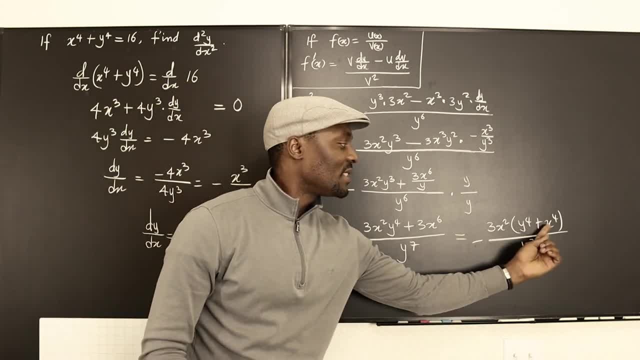 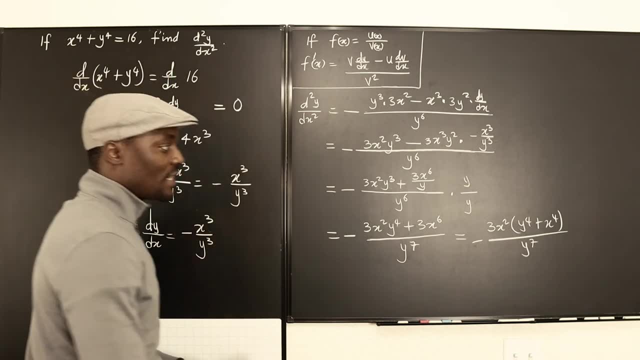 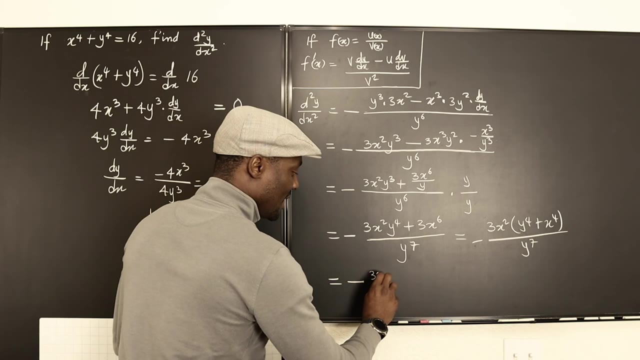 However, if you remember, y to the 4th plus x to the 4th was the question, And that was 16.. So I could go back here and put 16 here. Okay, So that means this expression is negative: 3x squared. 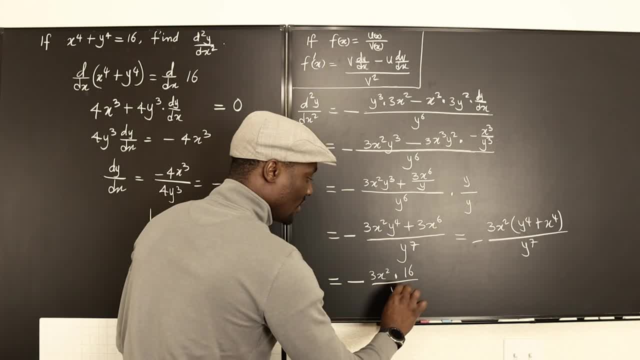 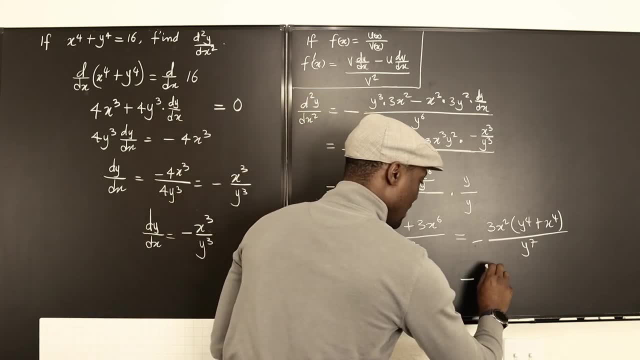 multiplied by 16 over y to the 7th, and that would give me negative 3 times 16 is 48, negative 48 x squared over y to the 7th, and that is the 2y dx squared.